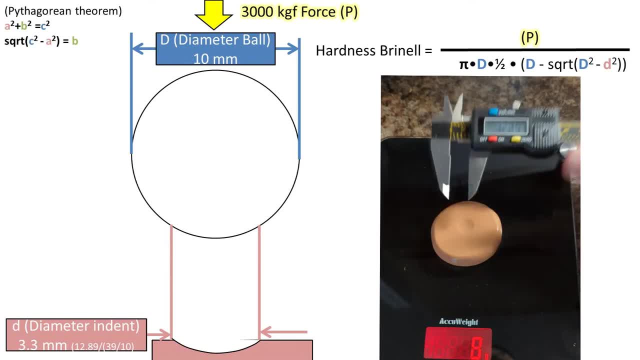 the indent diameter by 39 millimeters. over 10 millimeters We get 3.3 millimeter diameter for the indent. To reiterate, the only reason I'm scaling everything and changing the numbers is to match the standard weights and measures for a Brunel. 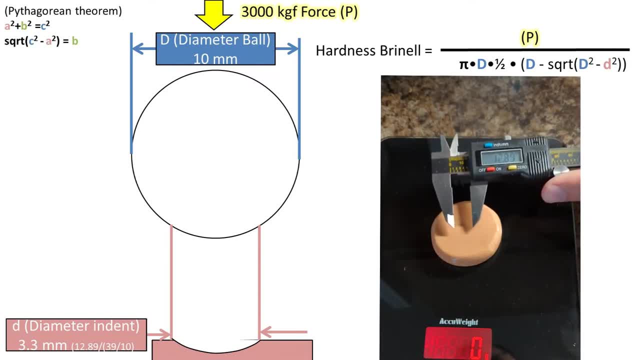 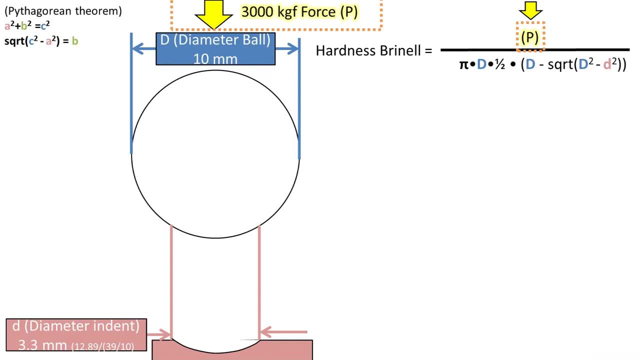 test. You would not really have to do this in reality, assuming you have the actual equipment. Also, my hardness number is going to be made up, So the Brunel hardness equation is the load, which typically is 3000 kg of force and is typically applied for about 30 seconds or so. 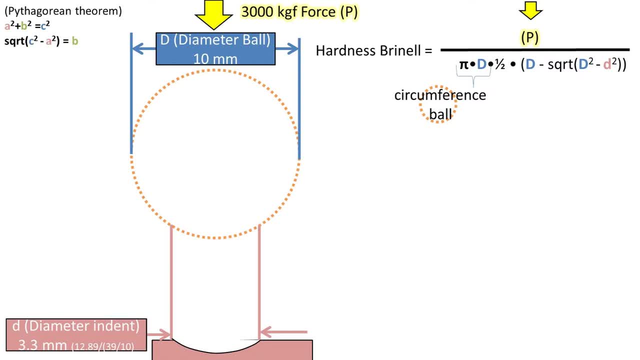 Divided by pi times the diameter, which is the circumference of the 10 millimeter ball, times one half the diameter of the ball, minus the square root of the diameter of the ball squared, minus the diameter of the indent squared. What is this section doing? 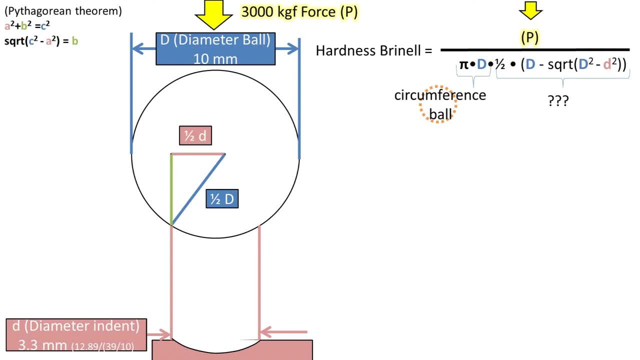 This looks like the Pythagorean theorem to me. so let's place a right triangle in the middle of the ping pong ball, with one lag being one half the indent diameter and the hypotenuse or longest side being one half the diameter of the ball used for this testing. Plugging these values into the 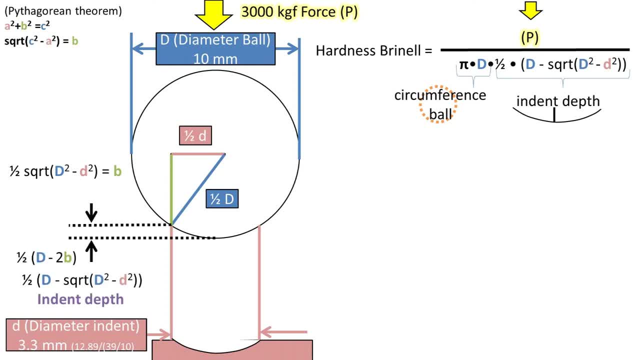 Pythagorean theorem, we get the other side length. Now if we subtract the side length from the diameter of the ball, we get the indent depth. so this portion of the equation is solving for the indent depth into the clay from the bottom of the steel indent sphere. So really the formula is: 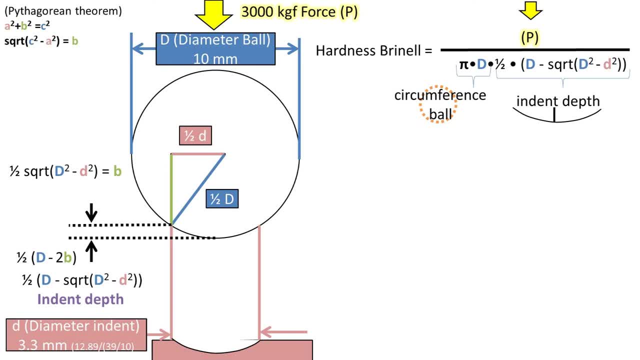 load divided by the circumference of the indent sphere times the depth of the indent. So let's plug in these numbers I made up and see what the hardness we get. We get a hardness of 340.9.. This, of course, is not an actual hardness, but if you were to get 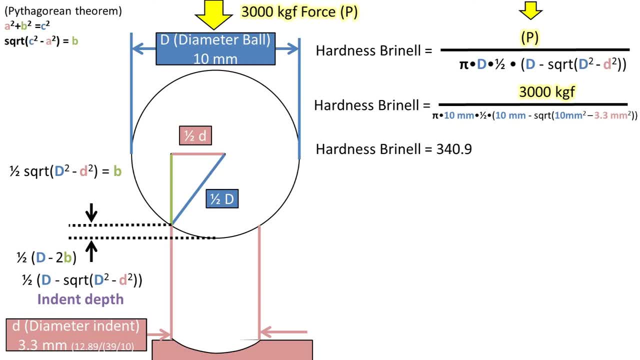 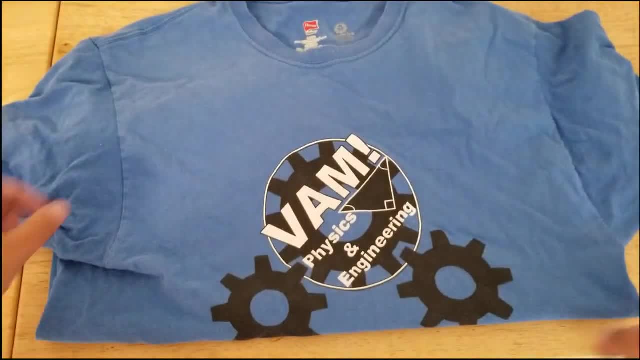 this value. you could compare it to experimental values to see how hard your substance is. Poll update. That concludes this video. Hope I've earned a like, share or subscription. It really helps me out the channel, if you do. If you enjoyed this video, you may enjoy one of these videos as well. 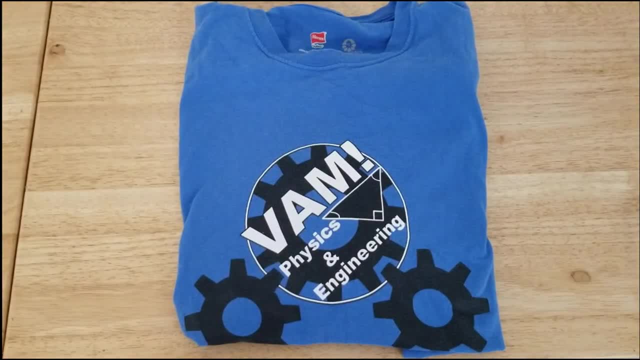 Let me know how I'm doing in the comments down below. Thank you for watching.